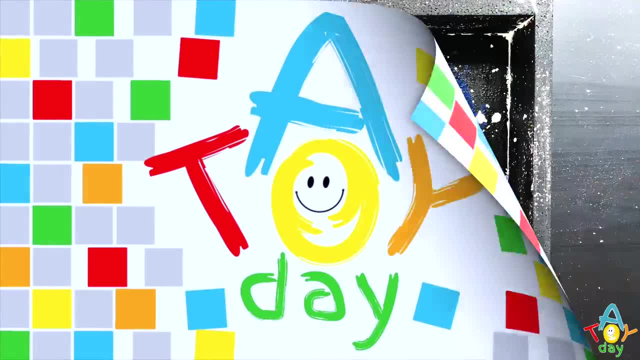 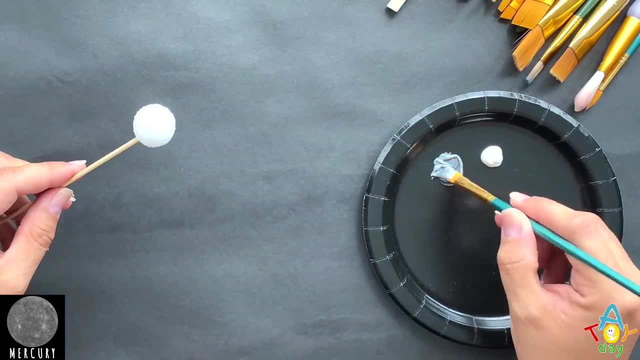 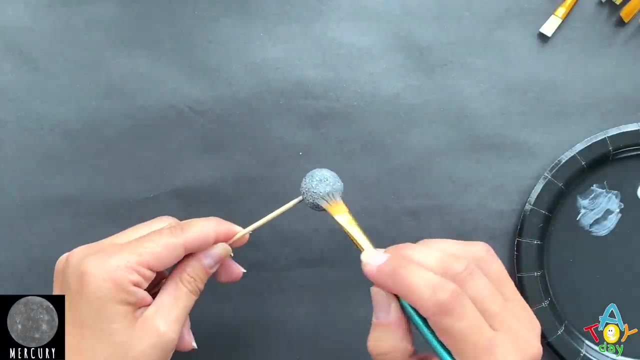 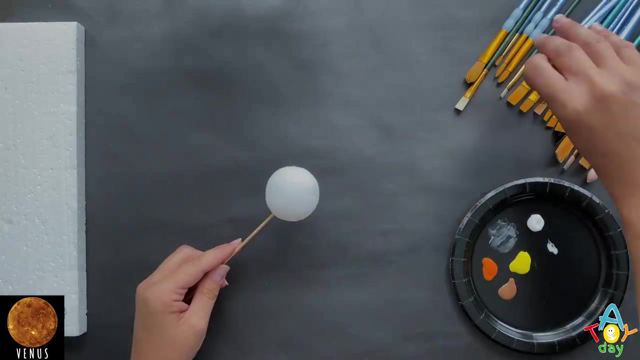 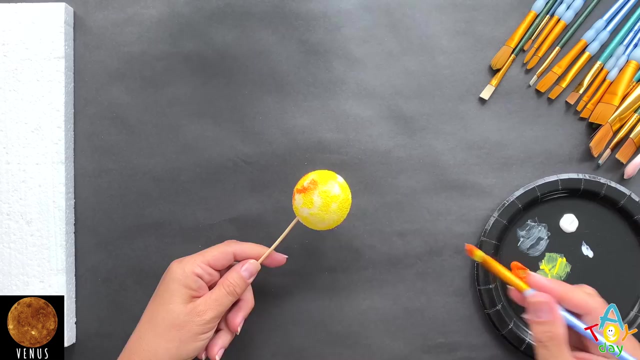 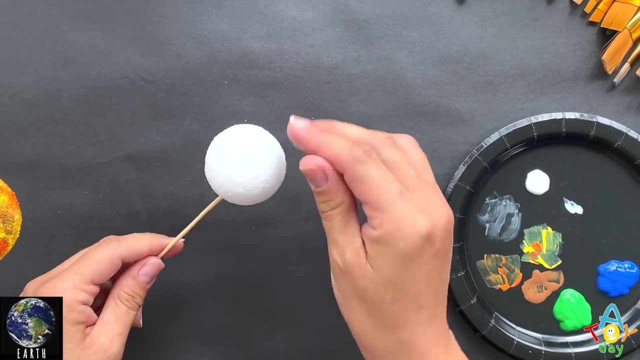 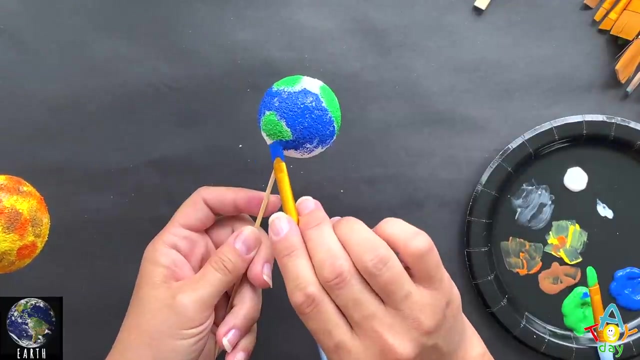 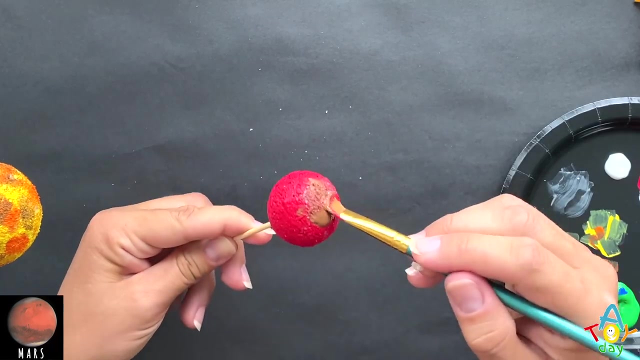 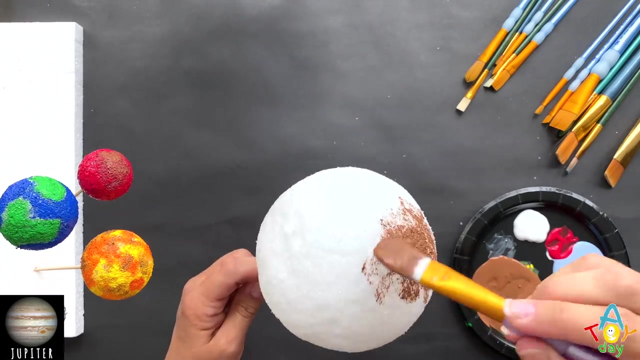 Please subscribe to our channel and press the bell icon to receive notifications when we upload new videos. Thank you for watching. Please subscribe to our channel and press the bell icon to receive notifications when we upload new videos. Please subscribe to our channel and press the bell icon to receive notifications when we upload new videos. 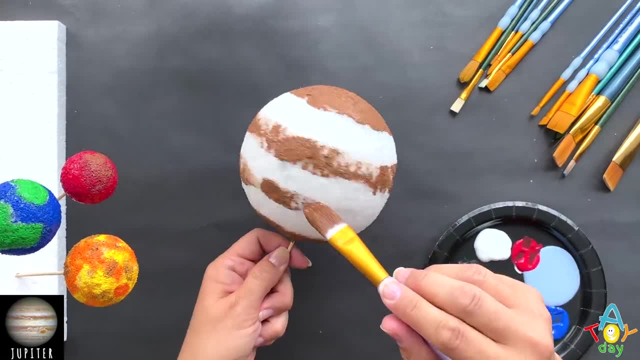 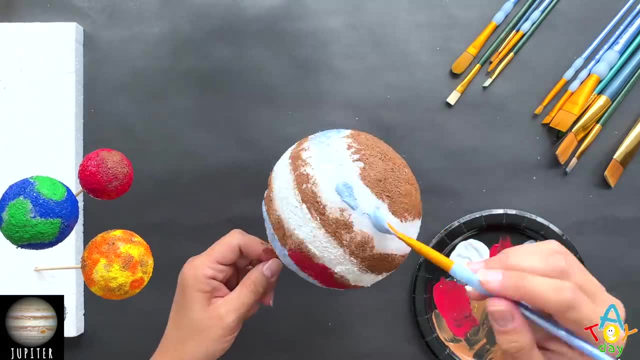 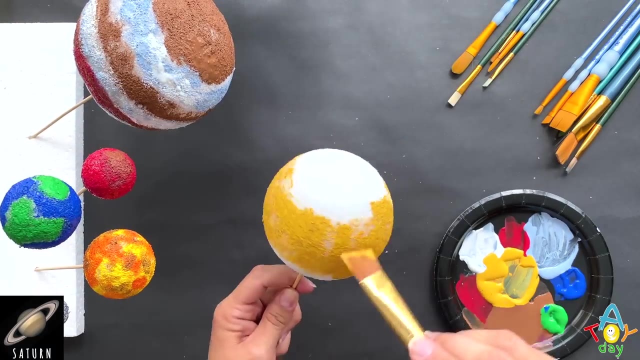 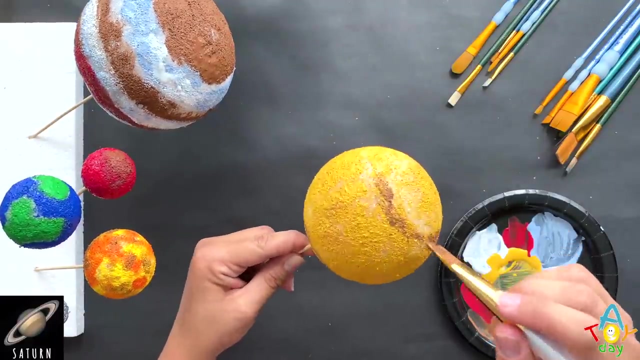 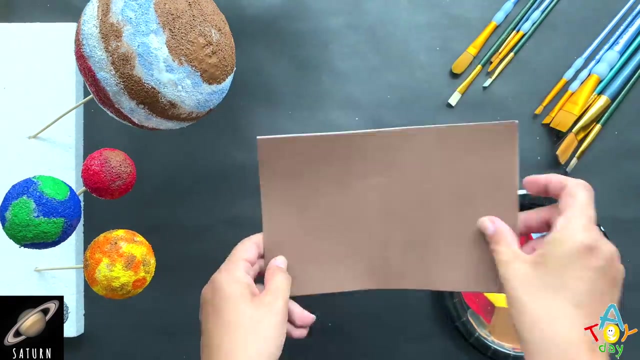 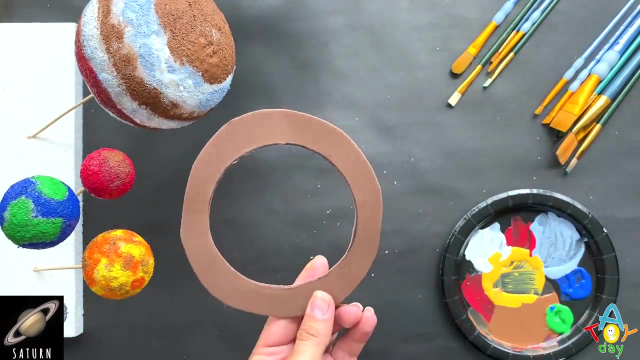 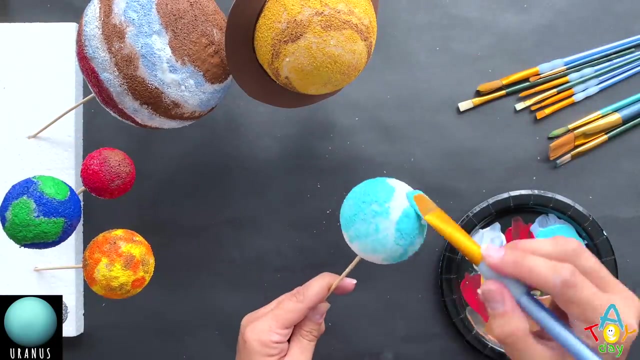 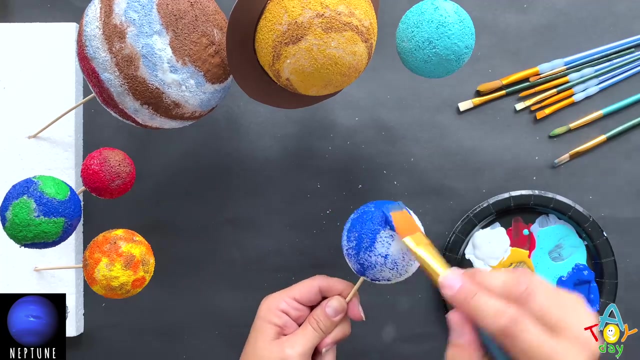 Thank you for watching. Please subscribe to our channel and press the bell icon to receive notifications when we upload new videos. Beat the�sx говорят at the l ads l es. You can see its beautiful rings, Uranus Ice giant which rotates on its side, Neptune. 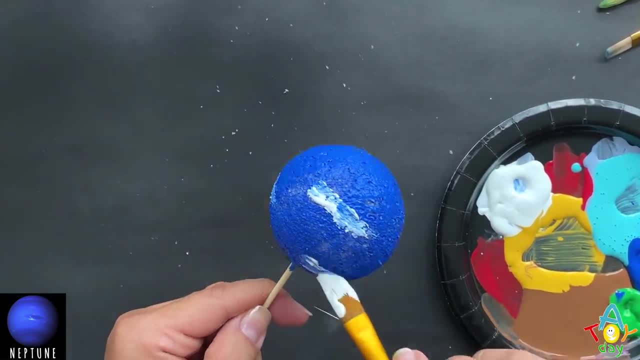 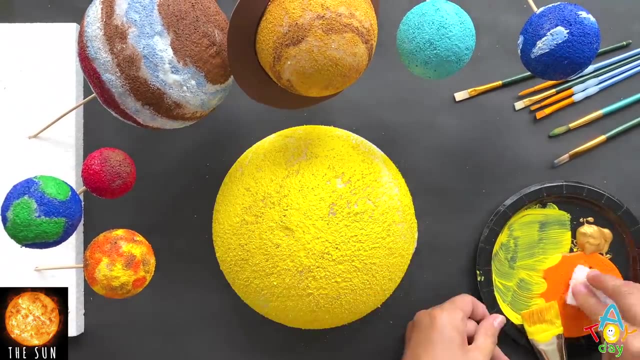 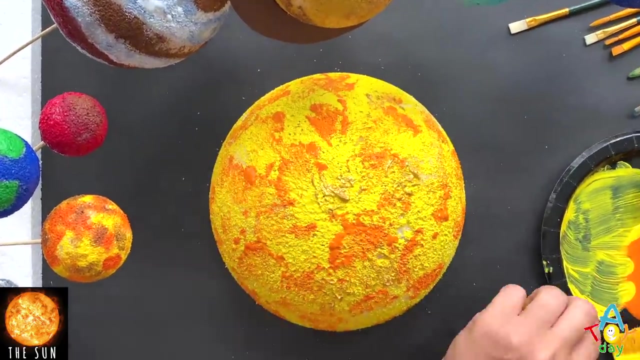 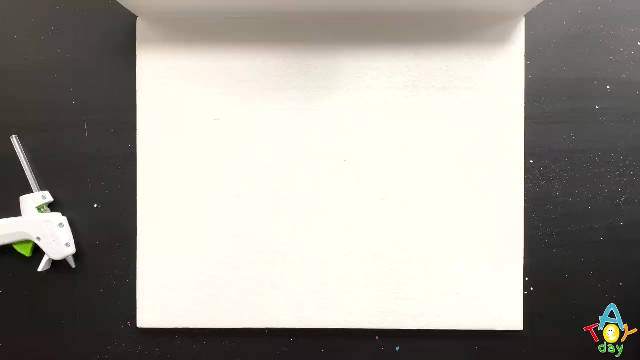 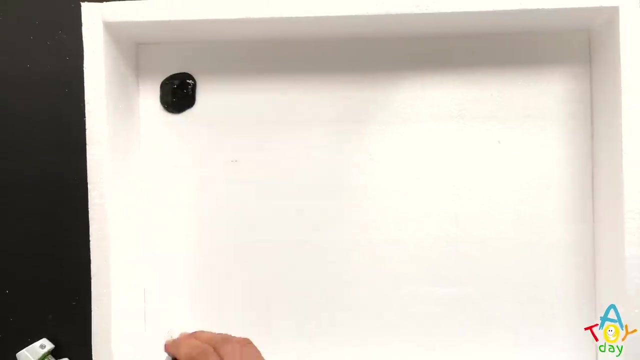 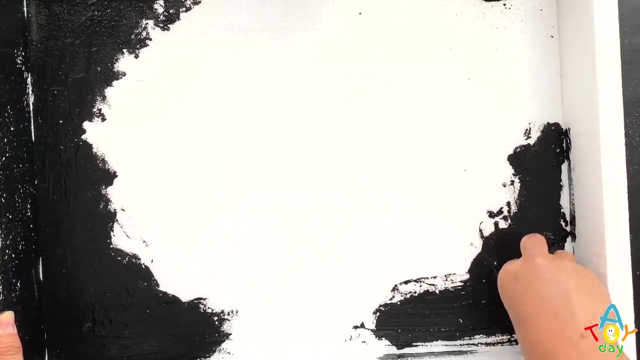 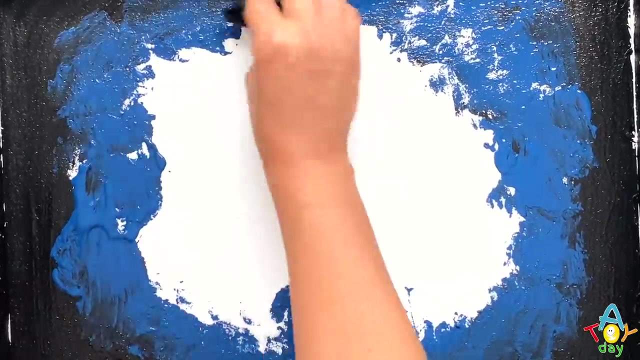 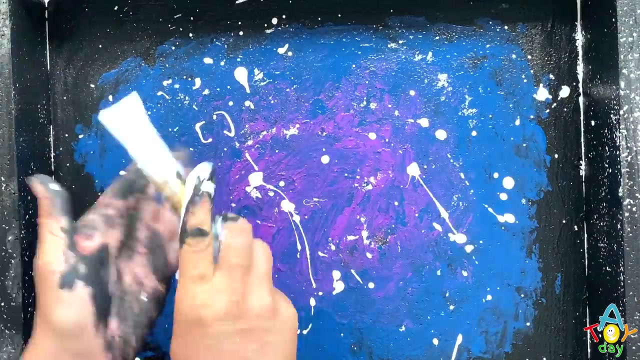 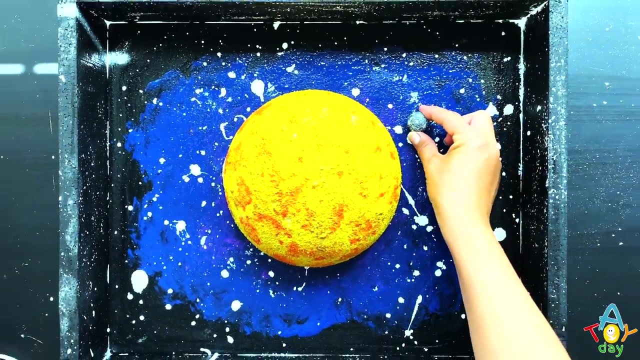